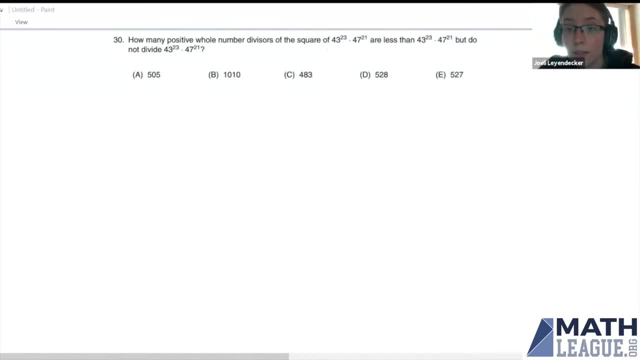 So, to get us started, the square of this number is going to be 43 to the power of 46 times 47 times the power of to the power of 42. Because you know to square it, we're just going to. 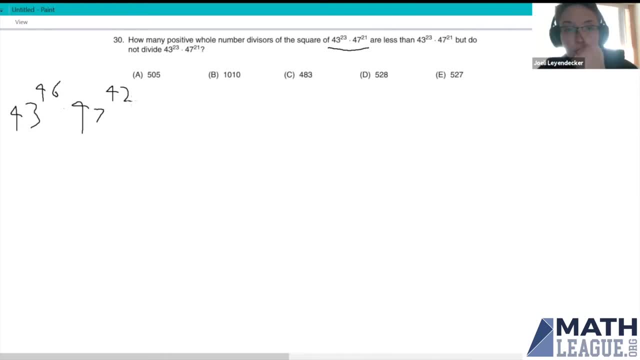 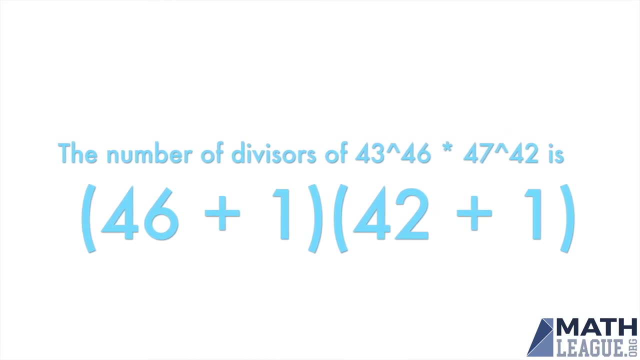 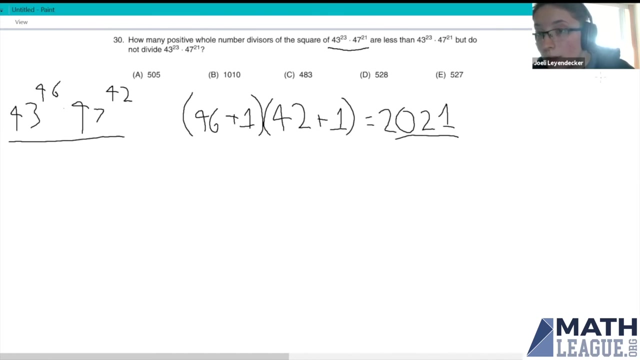 double the number of factors of each prime divisor of the number. So this number has 46 plus 1 times 42 plus 1 divisors, or 2,021 divisors. Now one of these divisors is going to be 43 to the power of 23 times 47 to the power of 21,. right, 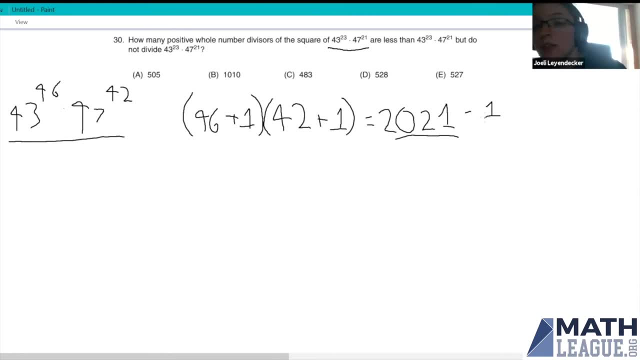 But so if we subtract that, because there's only going to be that one- that multiplied by itself gives us this number, We get 2,020 divisors that aren't this square or this number. And of these 2,020 divisors they can be paired up into factor pairs. 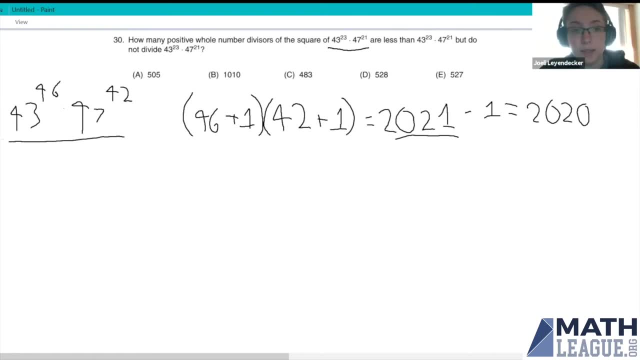 where multiplying one by the other gives us this number, And of each of those pairs, one of those numbers will be less than this number and the other will be greater than that number right? So dividing 2,020 by 2, we get 1,010 total positive whole number. divisors of this number. 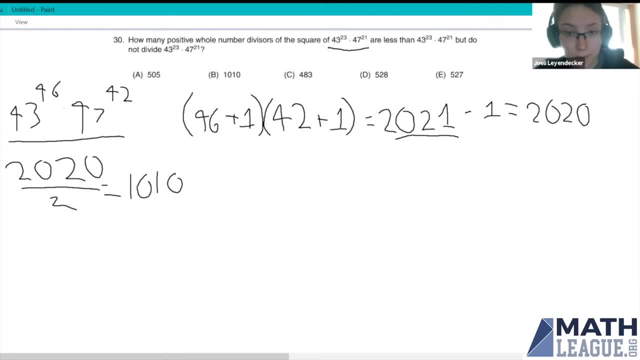 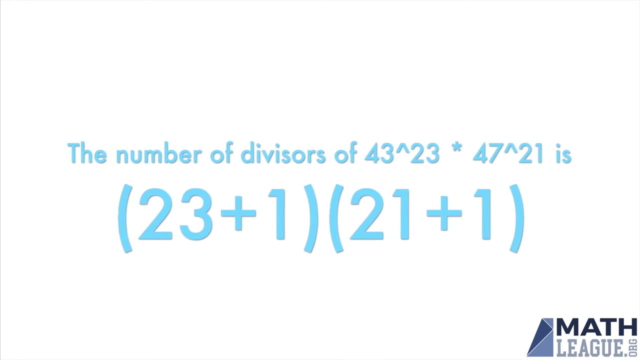 that are less than this number. Now, how many divisors does 43 to the power of 23 times 43?? How many divisors does 47 to the power of 21 have? Well, just like we calculated here, we see that this number has 23 plus 1 times 21 plus 1,. 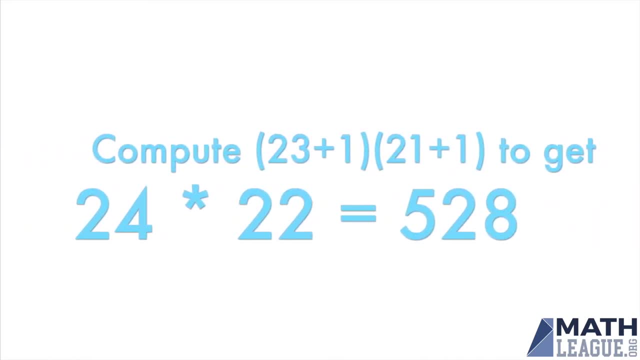 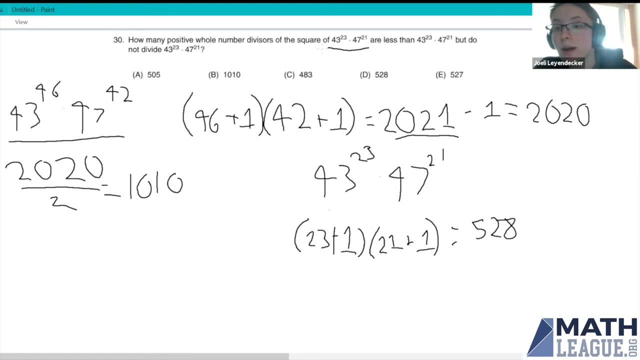 or 528 divisors. One of these divisors is going to be 43 to the power of 23 times 47 to the power of 21.. So the number of divisors that aren't equal, that aren't equal to the original number, is 527..